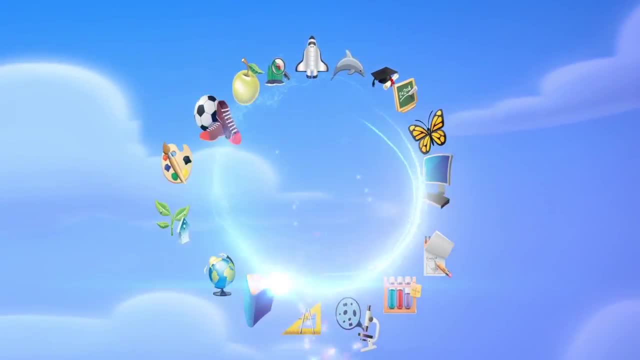 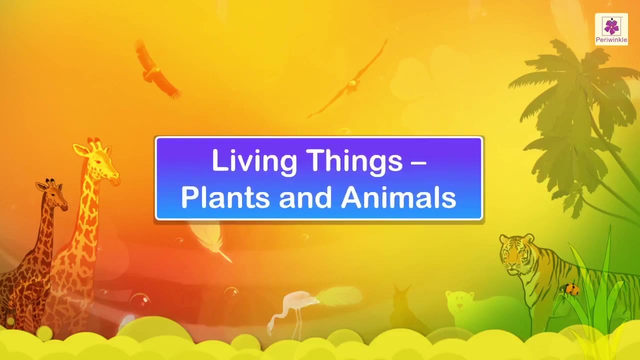 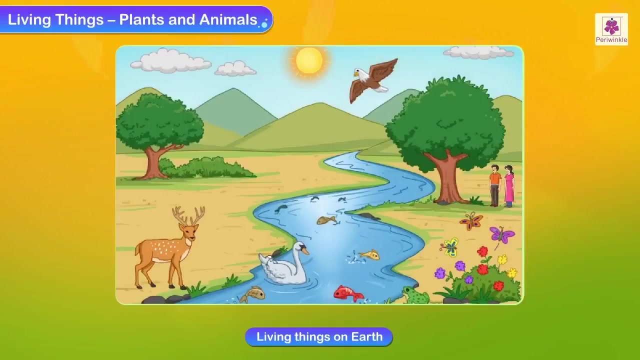 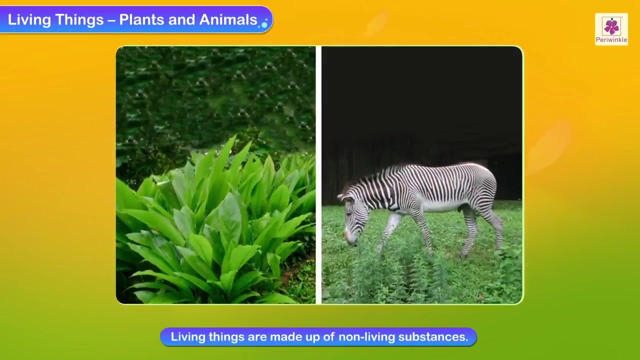 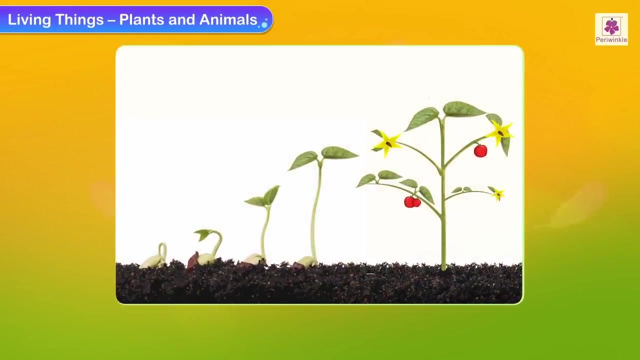 Living Things, Plants and Animals. Living things form the living world on the earth. They are a very important part of the natural environment. Living things on the basic level are made up of non-living substances. The natural things live in a delicate balance with the non-living things. 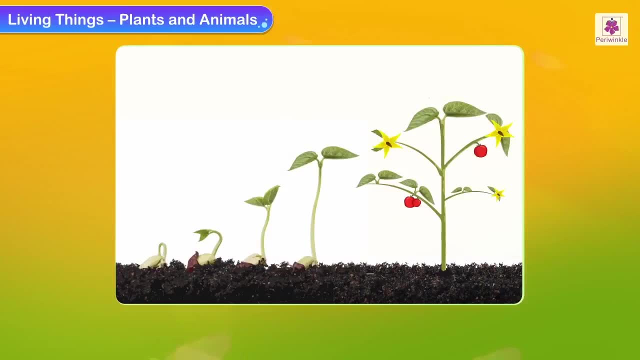 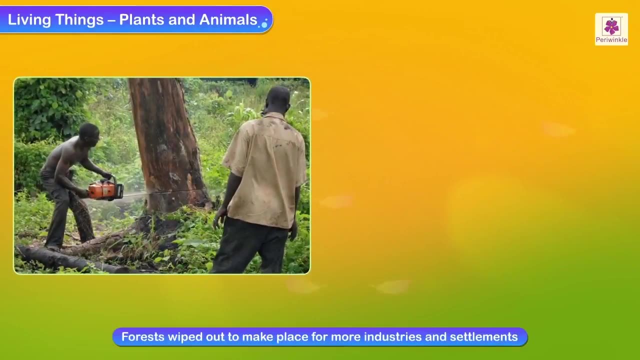 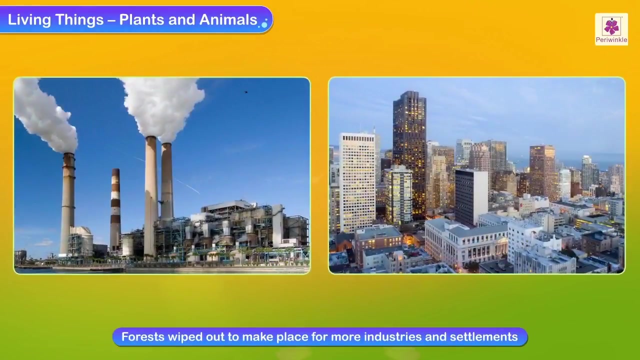 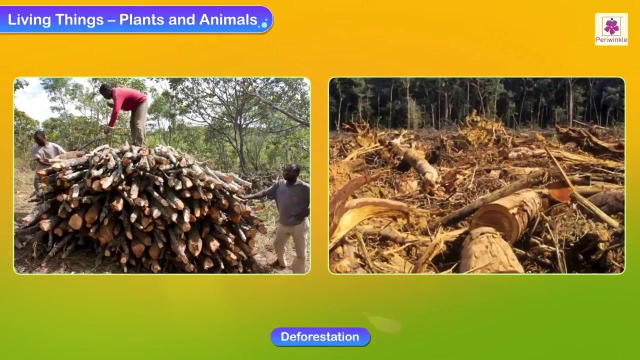 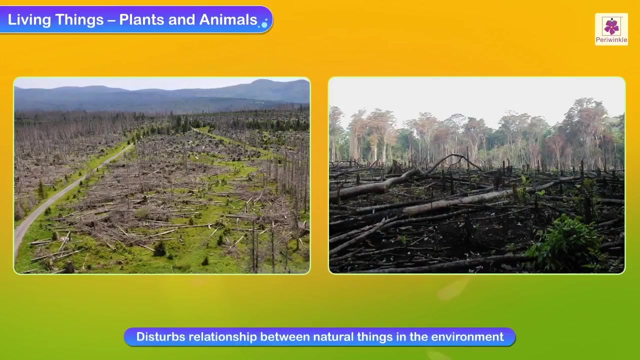 This needs to be maintained for the healthy survival of the earth. Man has wiped out forests In order to make place for more industries and settlements. This activity is known as deforestation. Deforestation has disturbed the relationship between natural things in the environment. 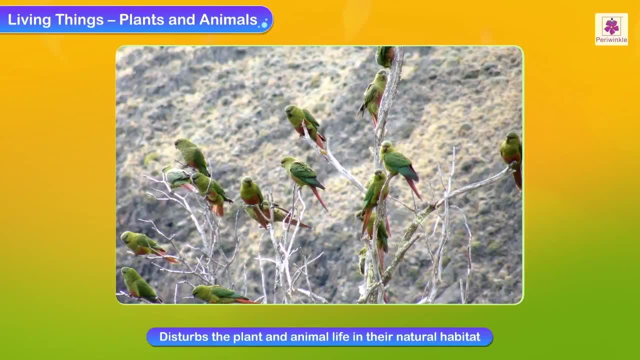 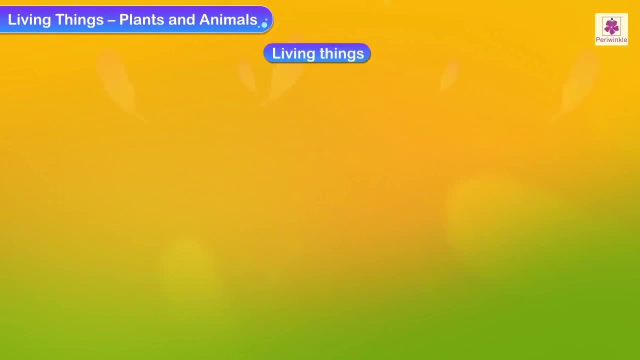 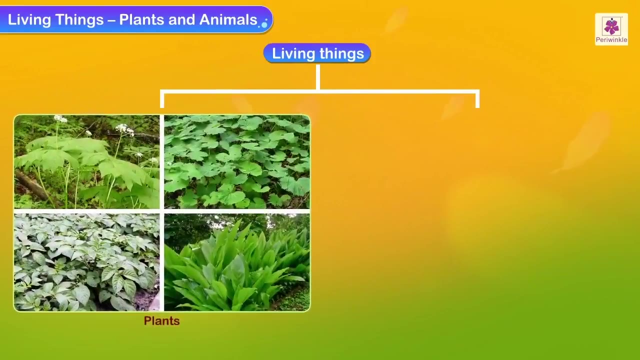 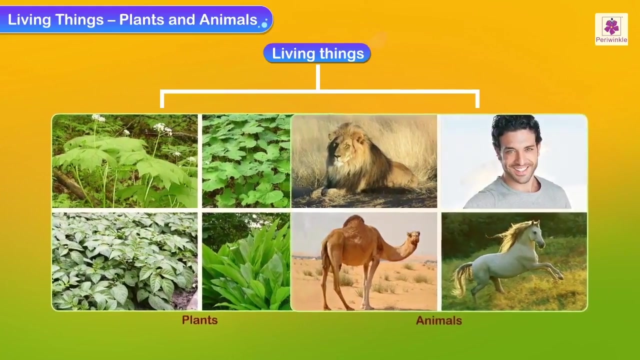 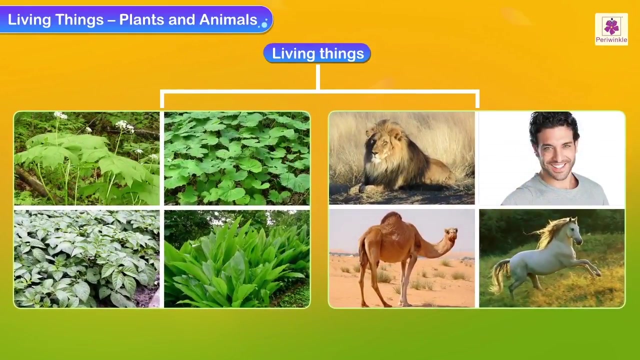 It also disturbs the plant And animal life in their natural habitat. Living things can be divided into two broad categories: Plants and animals. Although they both exhibit the characteristics of living things, They are different in many ways. Living things are different in many ways. 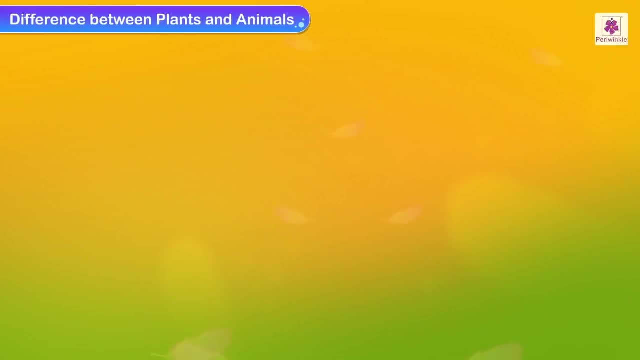 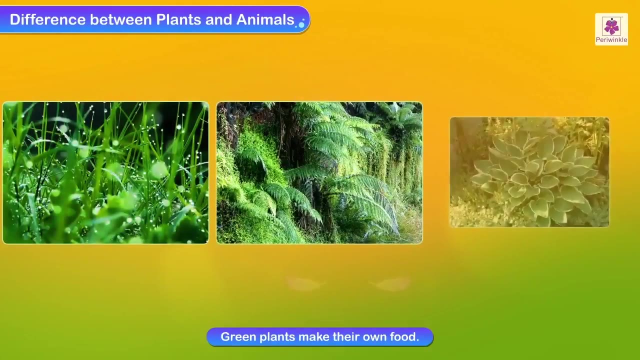 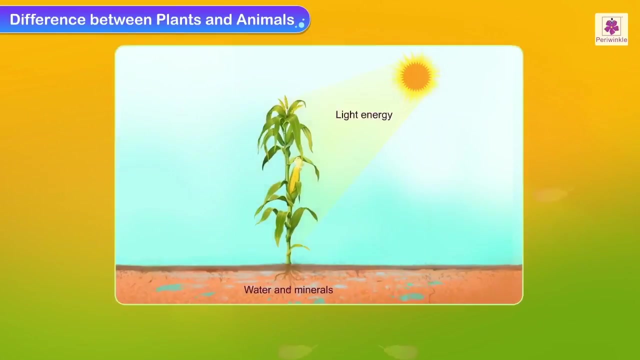 Above it, worlds will be組ed up in a particular tree. Living deals withLab and tea. They can also do other documents. They will next hugely influential things: Green plants: They make flowers, tea and water. Amidst thegunta of breeding plants, act in Ward birth. 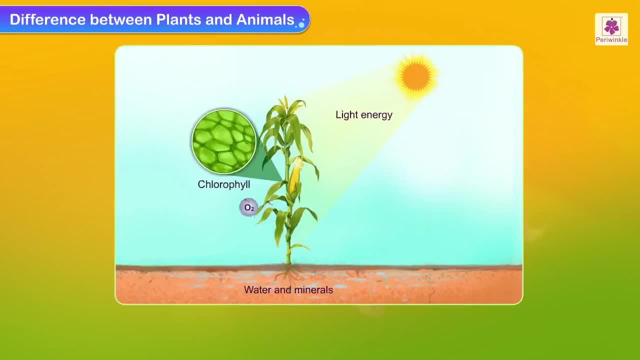 The difficult task is to help them канал. It is has two problems: The time of growing of plants. to defining Third Category, The duty of perfectly gumming plants. Want full control on the yield Food light that is required to make food for the plant. in presence of water and air, animals do. 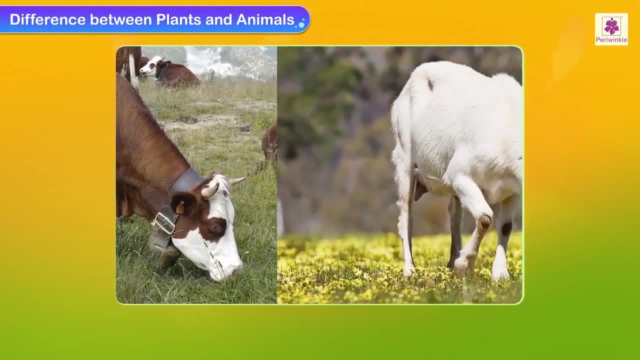 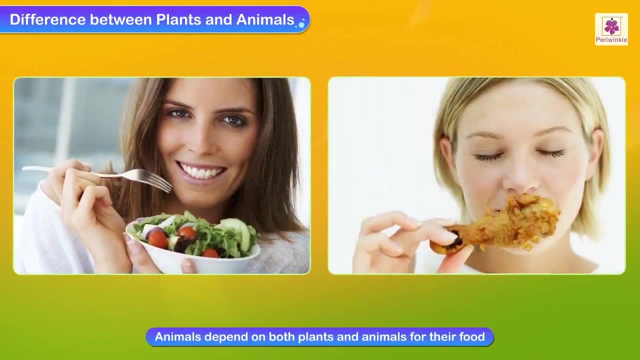 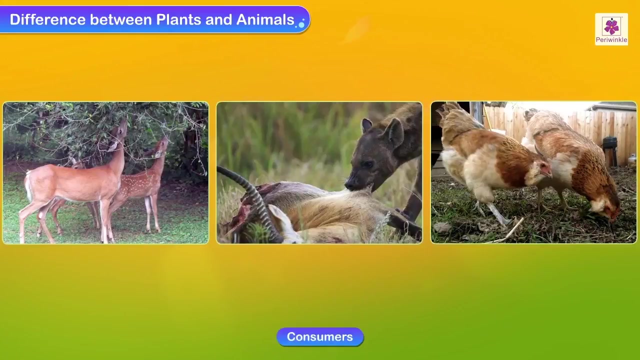 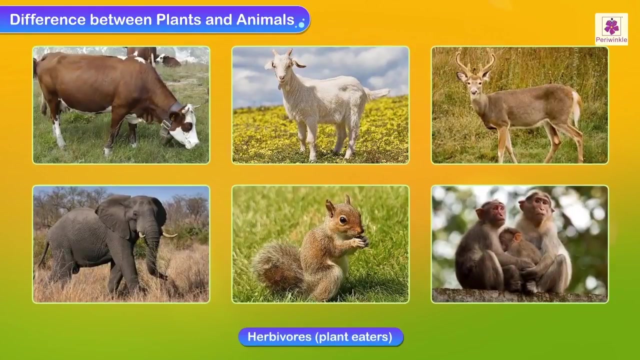 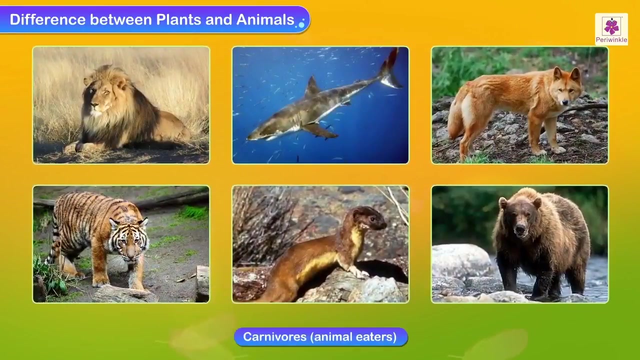 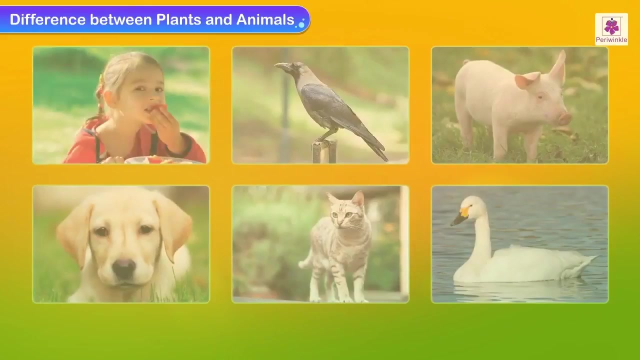 not make their own food, but depend on plants, other animals or both for their food. in general, they are termed as consumers. animals are either herbivores, that is plant eaters, or carnivores, that is animal eaters, living beings such as man, crow and some other animals. 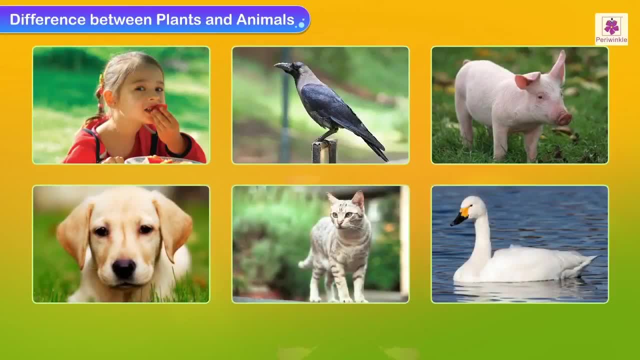 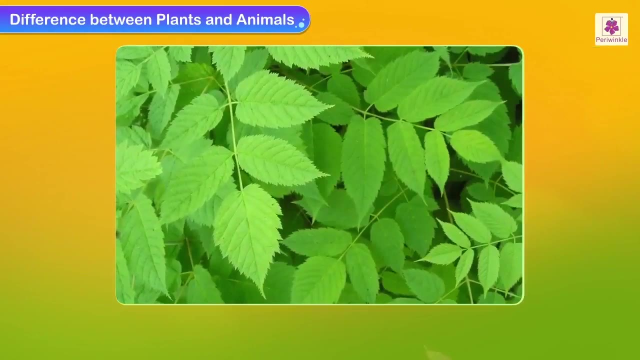 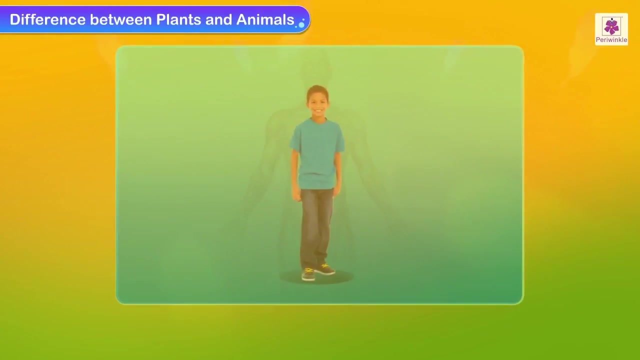 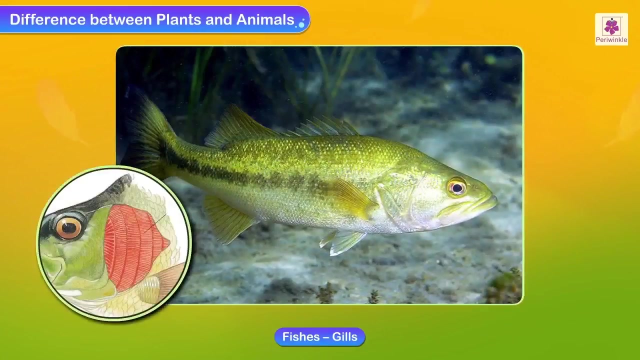 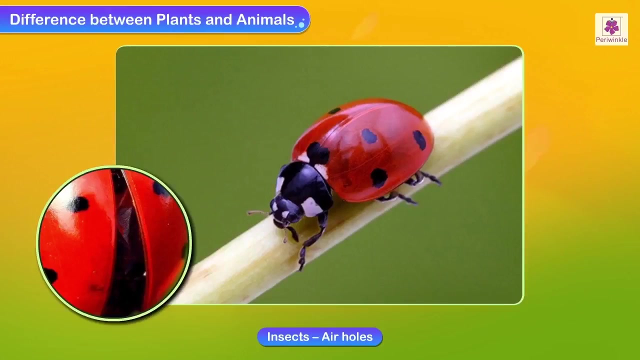 for feed on both plants and animals and are called omnivores, that is, both plant and animal eaters. plants take in air through tiny openings called stomata on the leaves. animals have different breathing organs. for example, man breathes through nose and lungs, fishes breathe through gills and insects breathe through air holes. plants show slow. 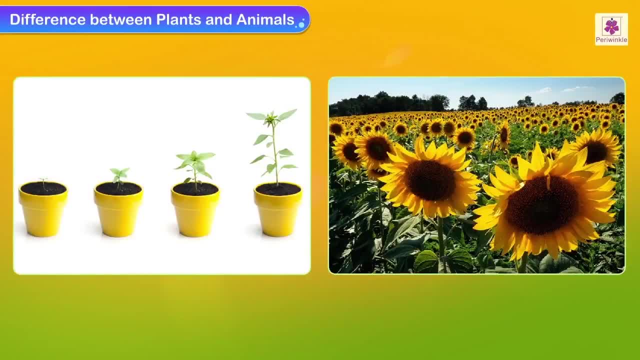 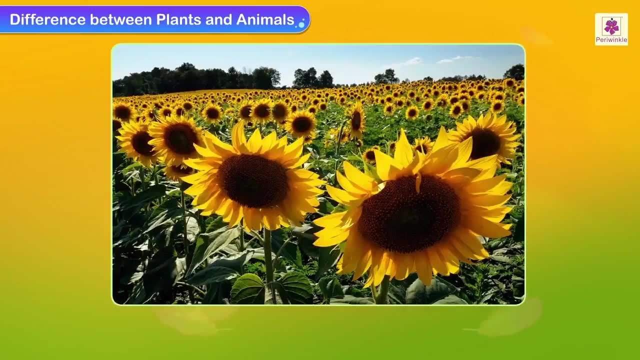 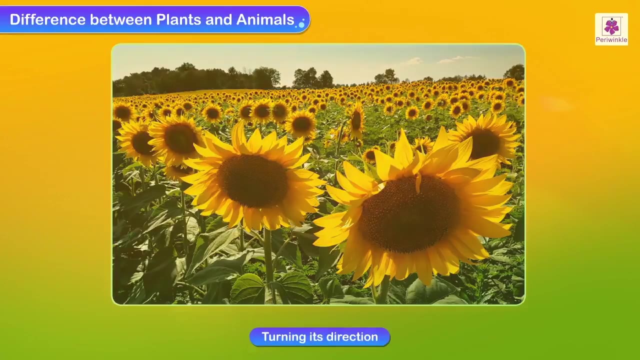 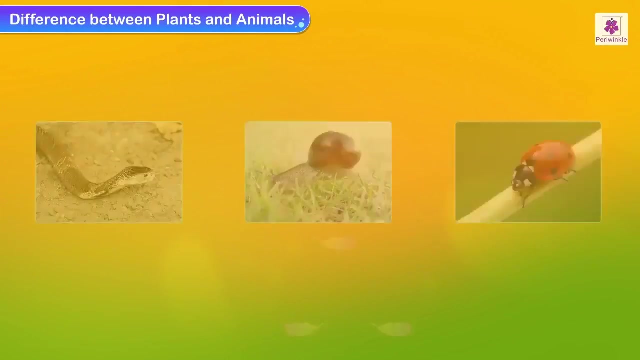 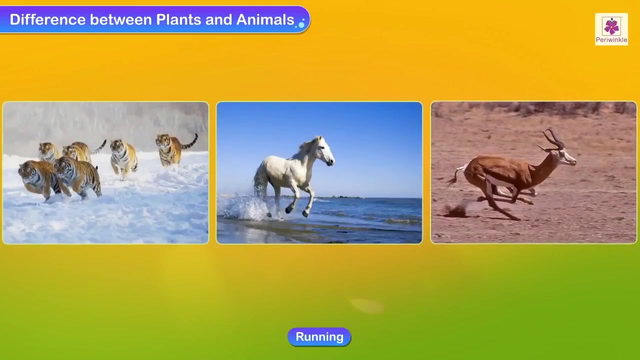 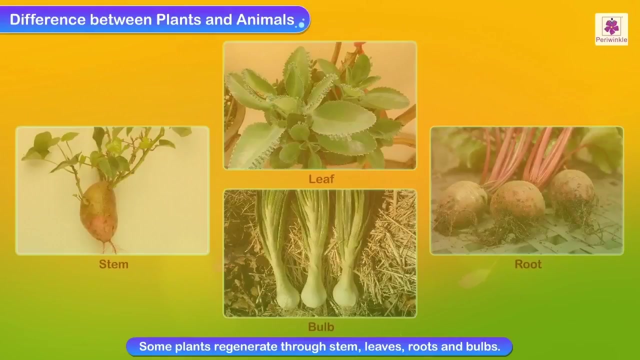 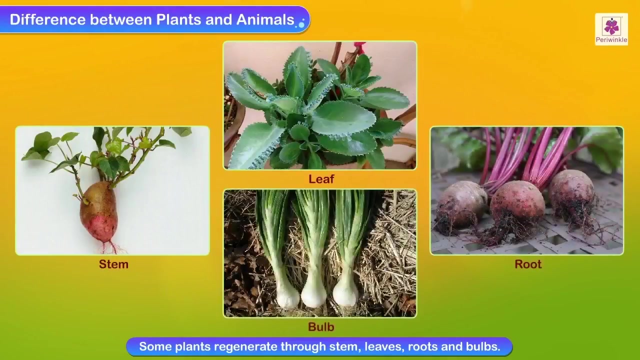 and subtle movements. such movements include growing. plants show slow and subtle movements. such movements include growing of shoots, flowers turning in the direction of the Sun, etc. animals show more visible movements like walking, crawling, hopping, running in search of food security and shelter. some plants regenerate through stems, leaves, roots and bulbs plants also. 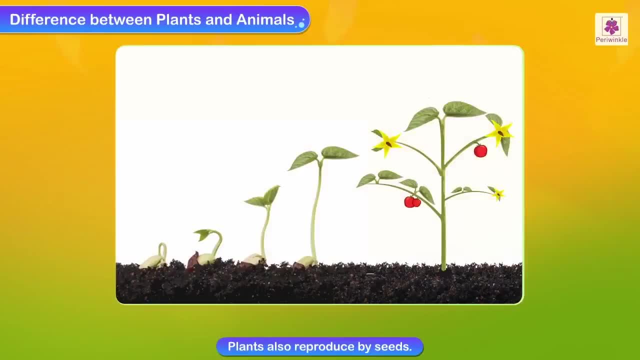 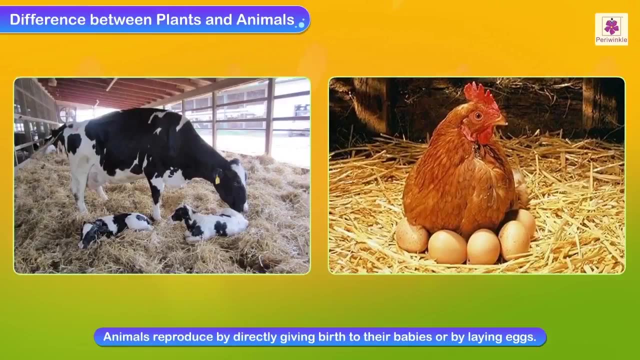 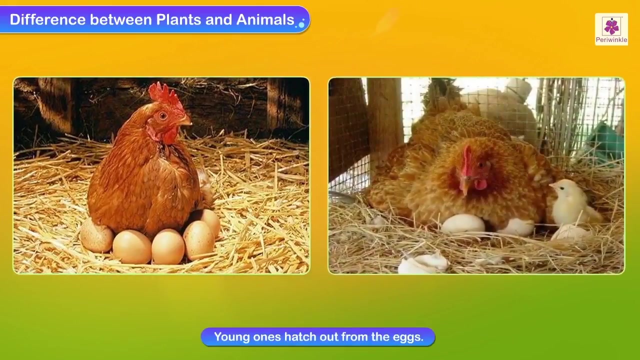 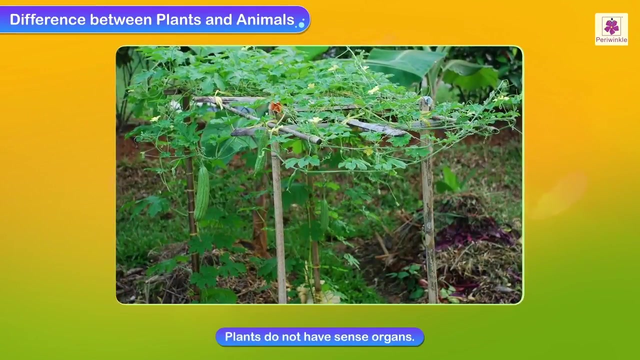 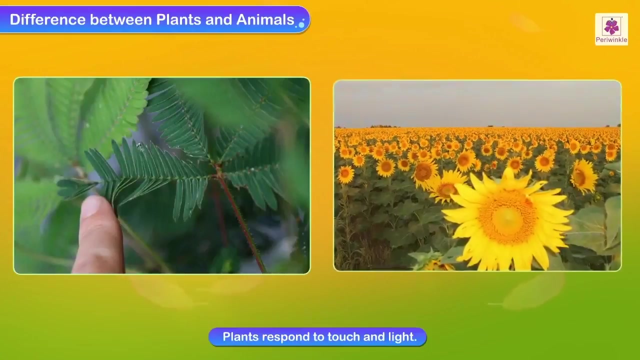 birds and bulbs. plants also reproduce by seeds. animals reproduce by directly reproduces by seeds. animals reproduce by directly giving birth to their babies or by laying eggs. young giving birth to their babies or by laying eggs. young hatch out from the eggs. plants do not have sense organs like the animals, but respond to touch and